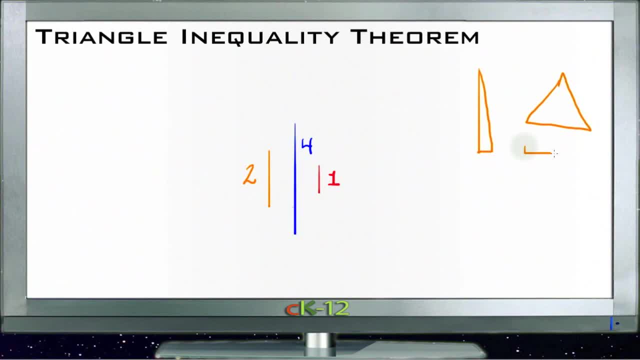 3, and clear on over to one that looks like this. that's way skinny in the other direction, So you should be able to just about make it out of any 3 different lines it looks like, But there is a limit. If you were to try and make a triangle where this side, here and this 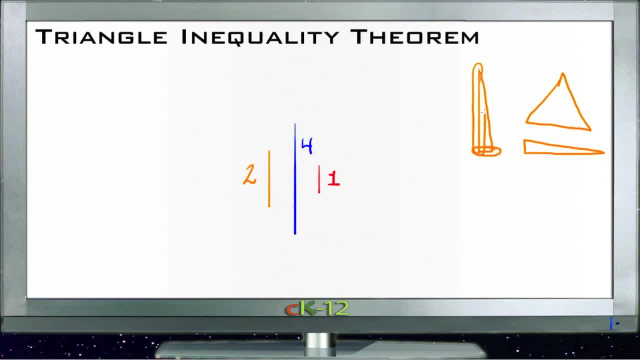 side here, for instance, weren't long enough added together to equal at least the third side, then those sides wouldn't touch, And you can see that here with my 3 lengths. If I try and make a triangle out of these 3 lengths, let's take this one here and we're. 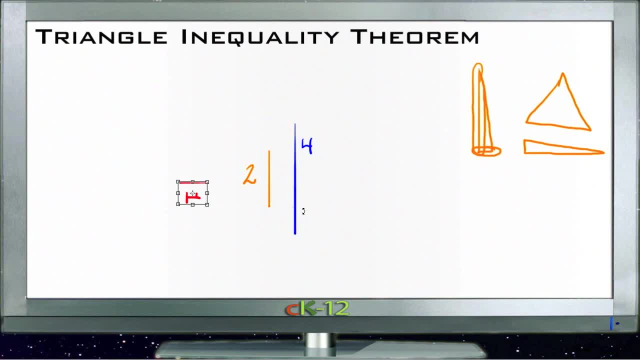 going to rotate it, so it's flat, and then we'll put: oh I don't know, let's move this one over here on the side, say we'll make this be our up-down side, move it into place there. there we go, and then we'll finally take this last one. We can see there's no. 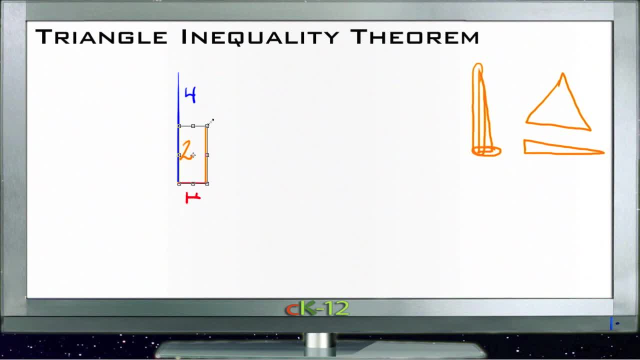 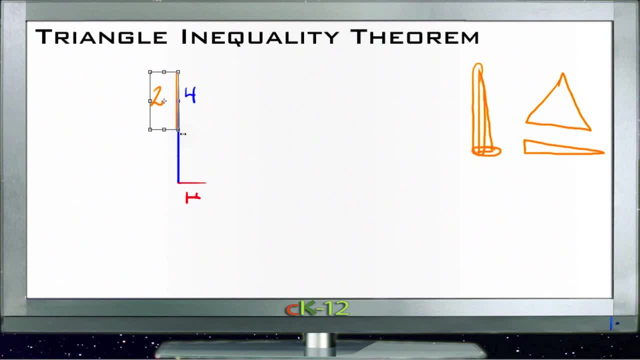 And even if I were to sort of set it up there and just barely barely angle it small as I can like, so there's no way that I can take side 1 and rotate it so that it's going to reach up there to side 2.. Again, no matter how tiny I make that, angle those two sides. 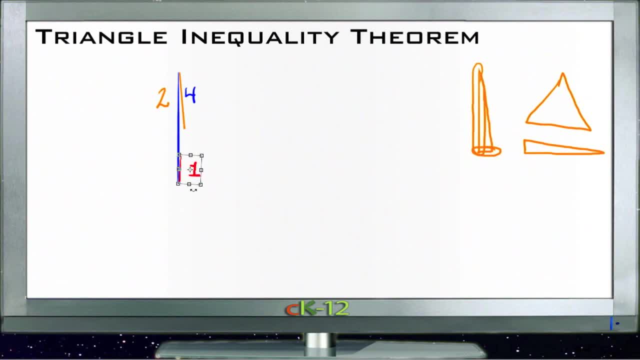 just aren't long enough to meet compared to side 4.. So there are limits to you know the sides of a triangle. If these two sides, if 1 and 2, if 1 plus 2 are not greater than. 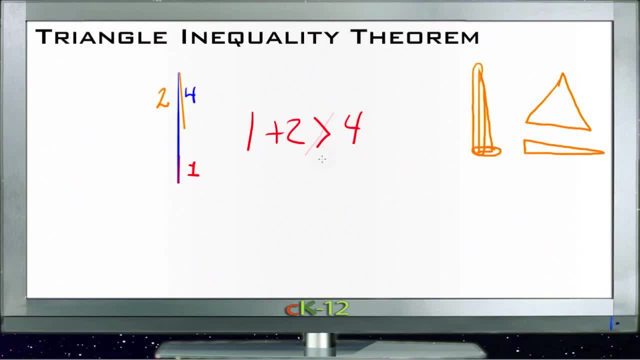 not greater than 4,, then it can't be a triangle. It can't be. If 1 and 2 aren't greater than 4, we can't make a triangle out of it, because these two not only have to be at least as 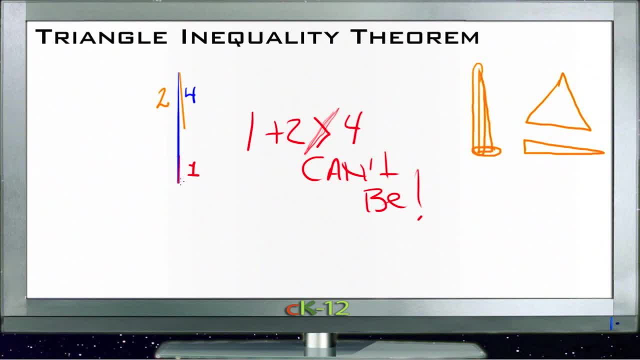 long as this, but they have to be a little bit longer so that they can sort of punch out the side this way and go a little further. And similarly, if I have two sides of a triangle, say, look a little like this, say and my 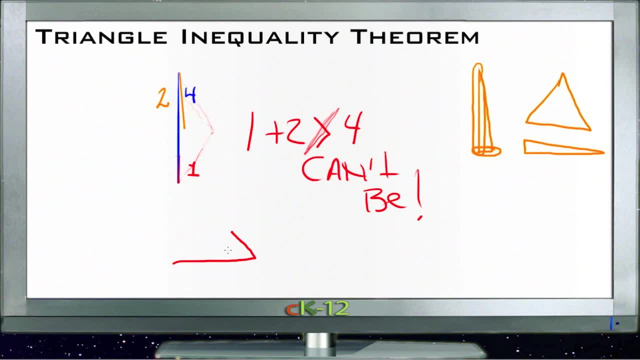 third side, the one I'm looking for, isn't at least as long as this difference between here and here. I still can't make a triangle. So if my third side over here that I'm trying to put in is, like you know, like this one here, 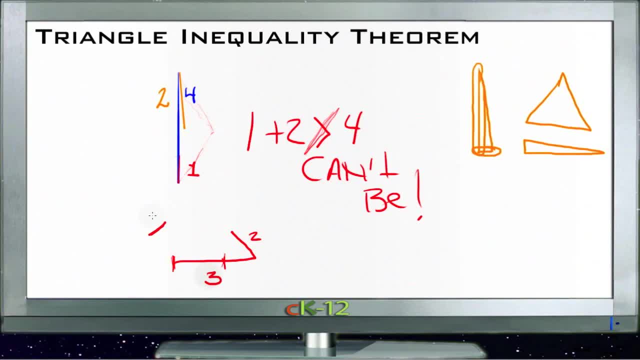 If we call this side 2.. 2 and 3 and this one 1, there's no way this side 1 over here is going to be able to make this into a triangle, because there's no way it's going to take the distance from this. 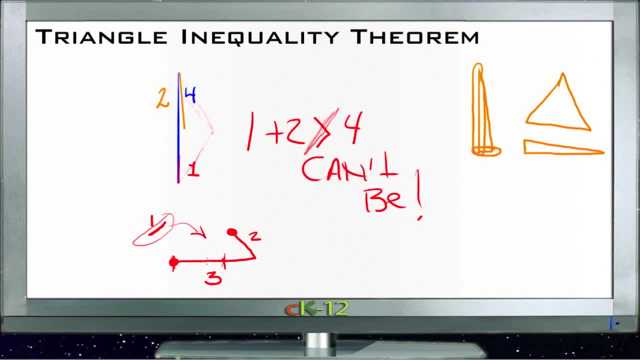 point to this point and connect them. So that's where that theorem that we talked about works. In order for a third side of a triangle to be the third side of a triangle, it has to be at least as big as the difference between the other two sides- 3 minus 2 in this case. so it has to be that big or bigger. 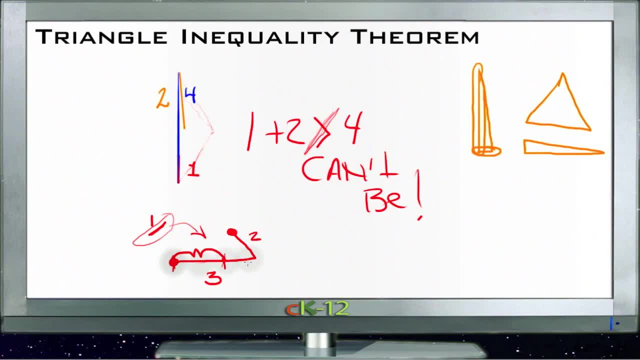 In fact it has to be bigger than that, Because if it's just that big, then you have a straight line, right. And it has to be smaller than, as we can see here. it has to be smaller than the other two lines added together. 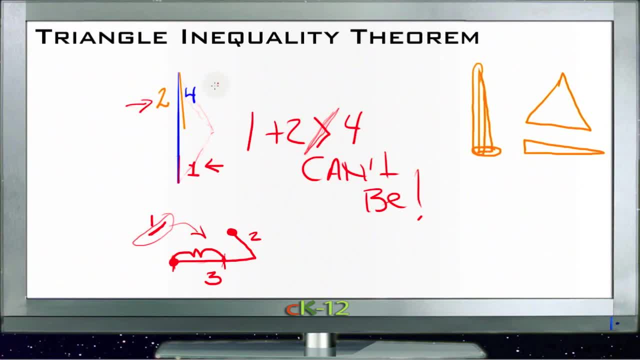 2 plus 1 can't be smaller than 4 or it's not going to work. So that's our triangle inequality theorem. Any side of a triangle has to be greater than the other two. we'll call those a and b? a. 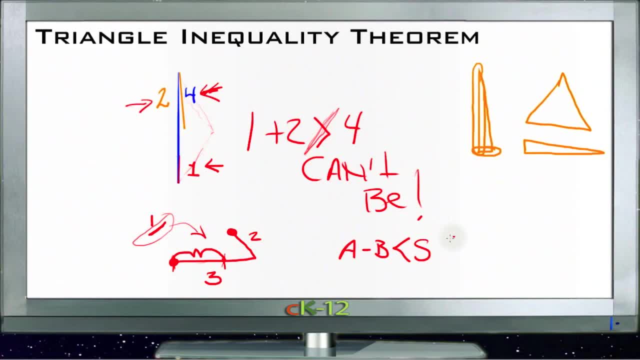 minus b. The difference has to be greater than the difference between the other two, But less than the other two combined. So a third side of a triangle- and often that'll be c if you like- third side of a triangle has to be greater than the difference and smaller than the total. Let's see how that applies to our example questions.